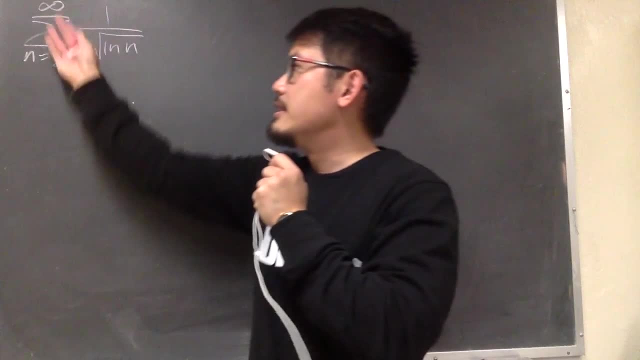 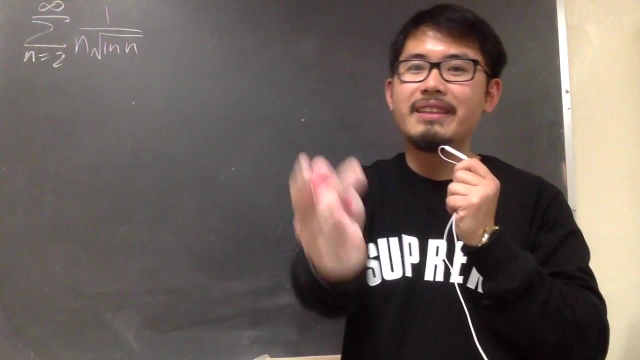 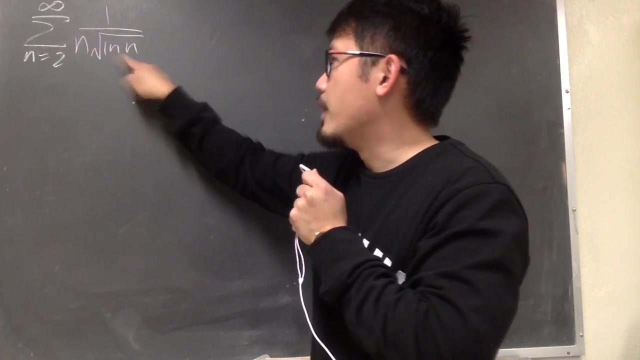 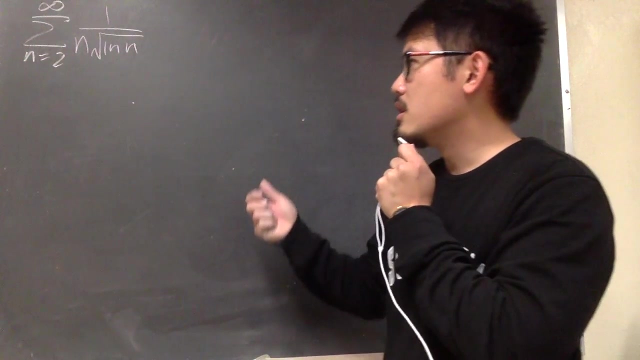 Maybe there's a good reason why, but then we'll focus on if this series converges or not. But sometimes the starting value doesn't matter, except for the reason that you're going to tell me okay. Anyways, if you look at this, 1 over n times square root of ln- n, it's hard to do anything in the sense of doing the comparison or the ratio test or the root test. 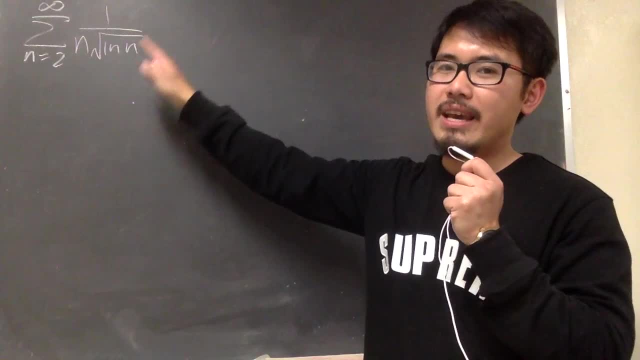 But it seems like this is something that we can integrate. If you look at this as 1 over n times square root of ln- n, it's hard to do anything in the sense of doing the comparison or the ratio test or the root test. 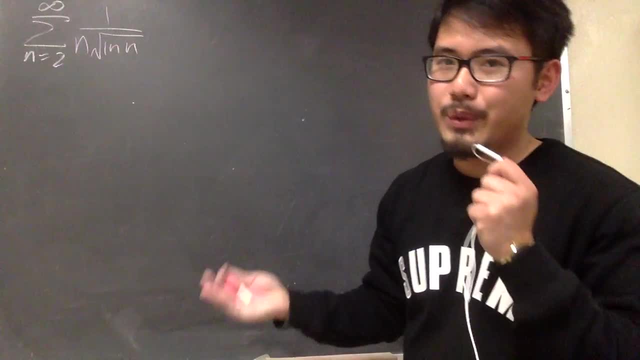 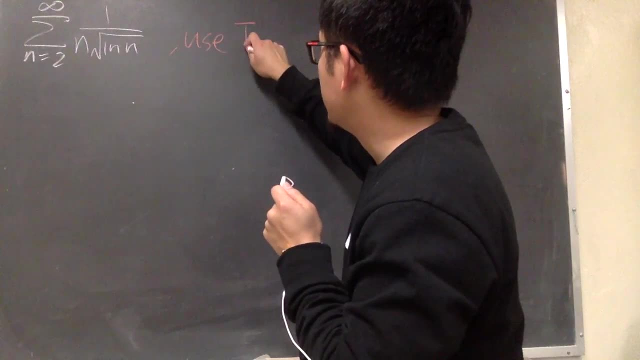 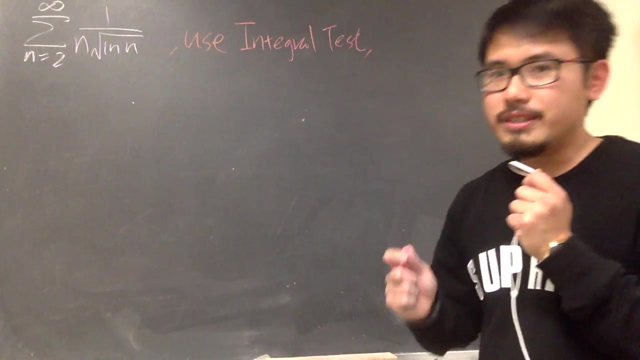 So 1 over x times square root of ln x. that's something that we can integrate With. that being said, let's use the integral test. Okay, so let me just indicate this: let's use the integral test And then, in order for us to use the integral, you have to tell me what the function is. 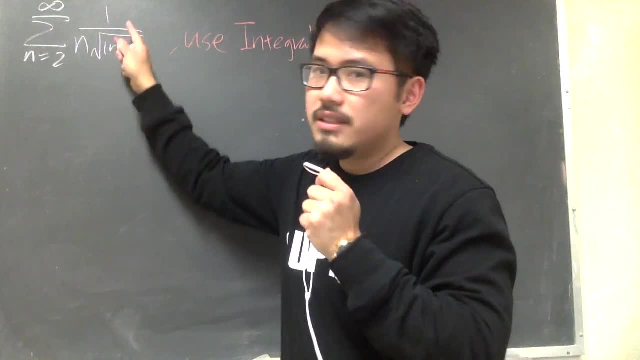 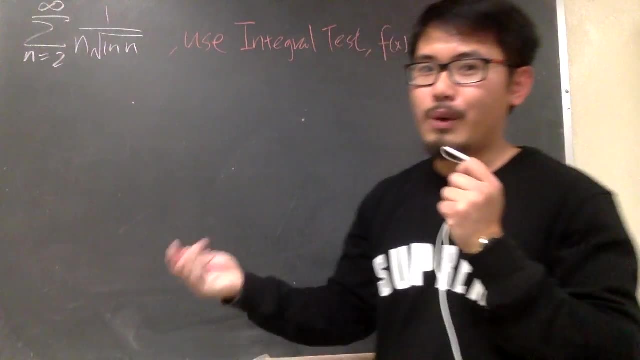 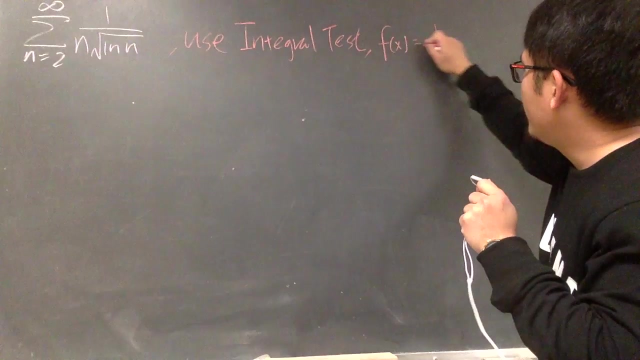 Of course, the function is just this, and you replace all the n with x, except for this n, that's the name ln. But then you replace: this become x and that become x. f of x is 1 over x times square root of ln, x. okay, And then, in order for us to use the integral test, 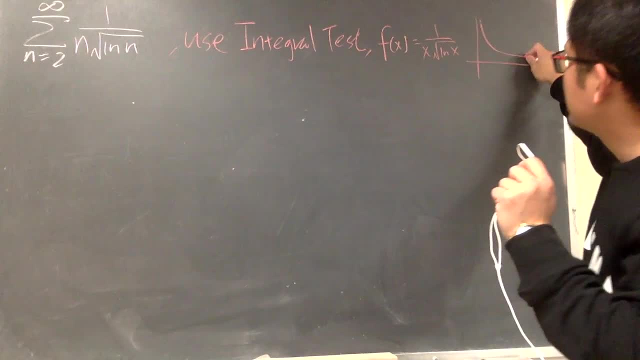 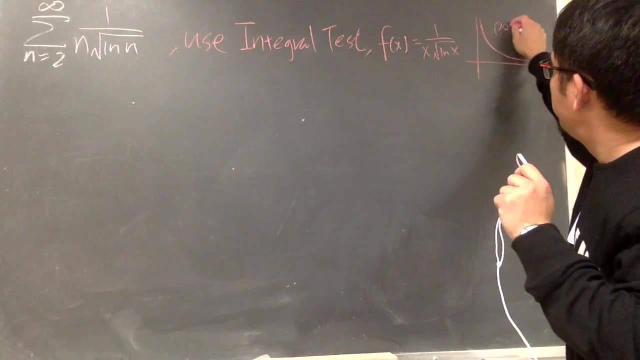 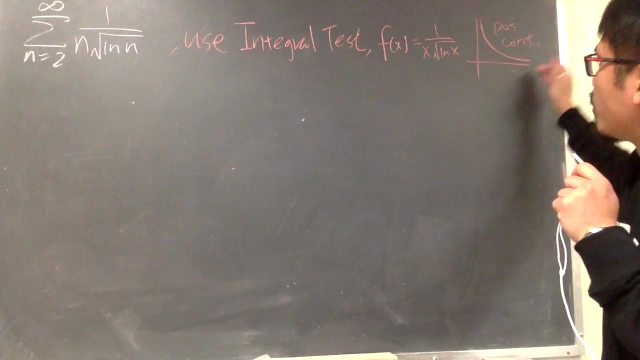 for this function we have to make sure three things. You can do a graph and you can tell me the three things. First, this function is positive, meaning it's above the x-axis, And second of all, it's continuous right for this portion. And then, third of all, it's decreasing. So I'll just 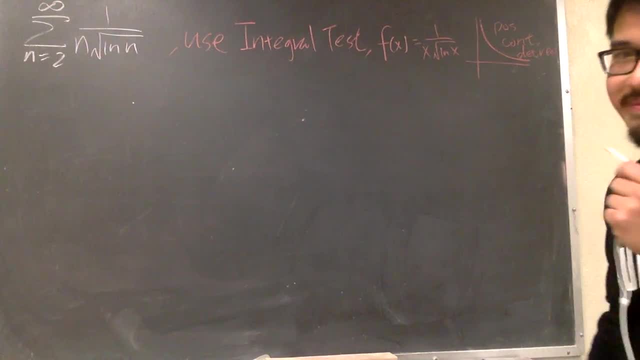 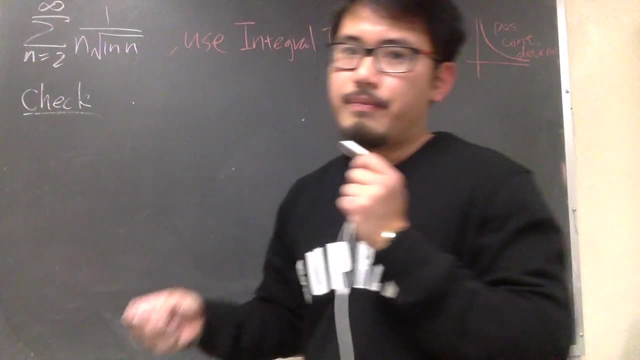 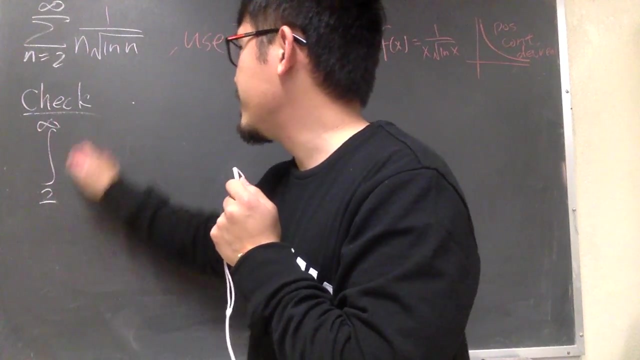 abbreviate this right here: decreasing. Yeah, Anyways, this is how it goes. I'm going to check the improper integral version of that. So let me work out the integral with you guys. From 2 to infinity: 1 over x. square root of ln x. 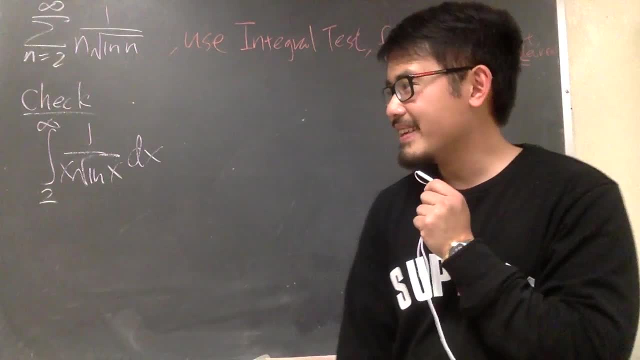 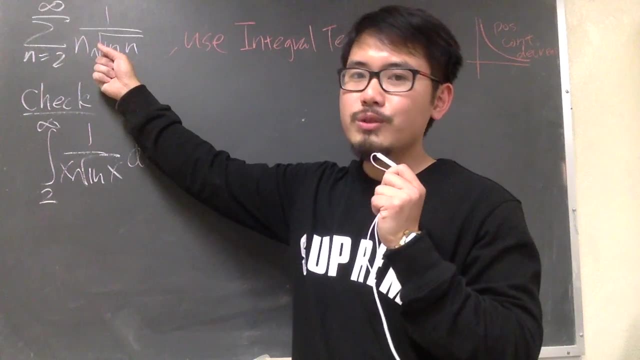 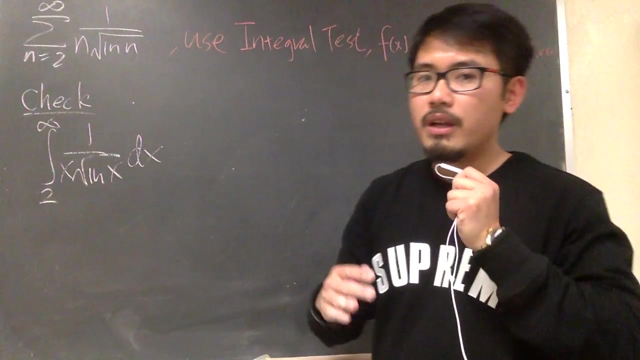 Haven't done integral for a while, right, All right. The integral test says: if this improper integral converges, then this right here also converges. If this diverges, this also diverges. But then in terms of the convergent, if this converges to 5,, for example, this does not. 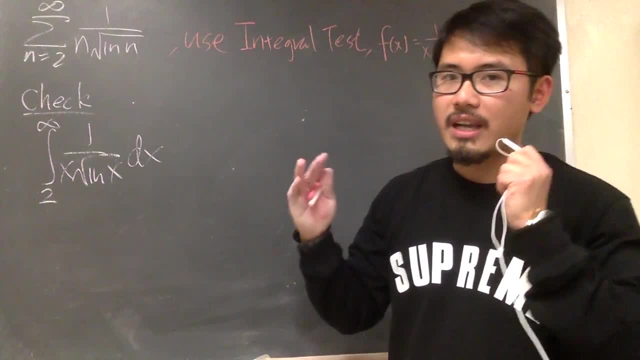 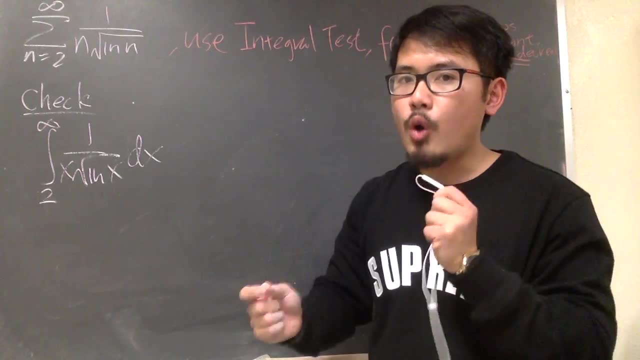 converge to 5. We only know in terms of the convergence. they will have the same convergence, Either they both converge or they don't. So we have to make sure that we have the same convergence. Either they both converge or they both diverge. They don't necessarily converge to the same value. 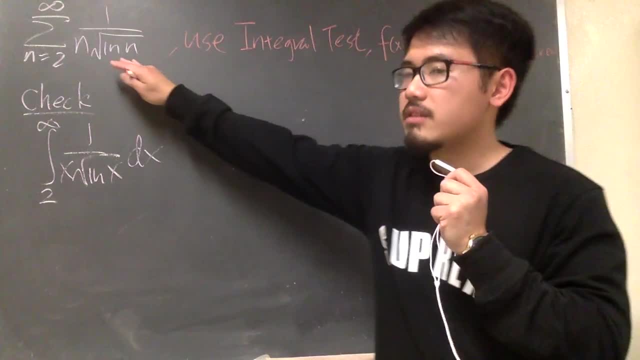 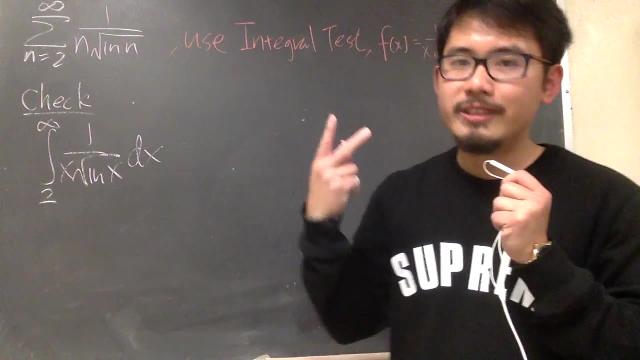 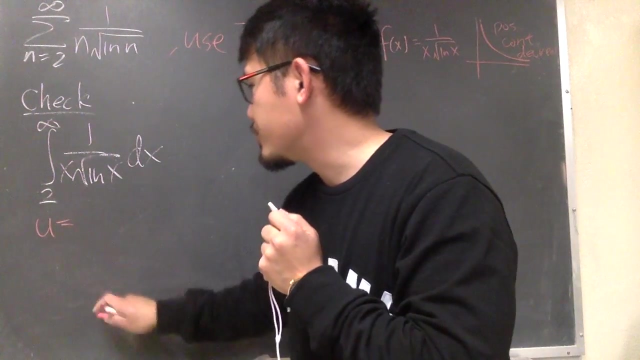 But then our answer: we only worry about if this converges or not. okay, All right, To do improper, integral two things: Know your integration and believe in your limit, So let's do it. To integrate this, I'm going to use the u substitution that u equals to inside. 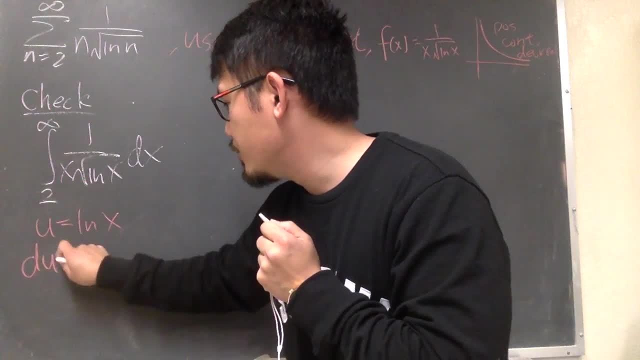 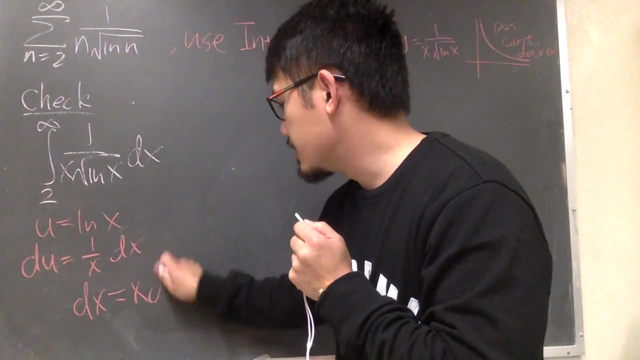 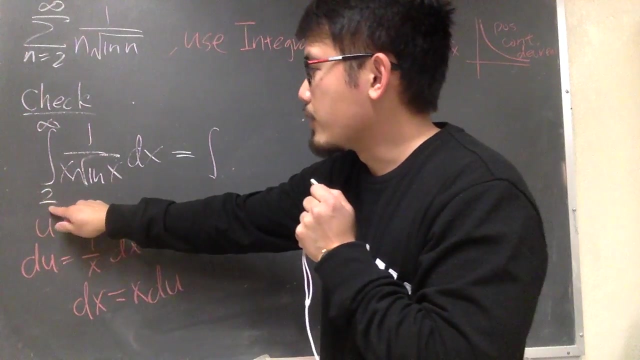 function which is the ln x. And then you see, du is 1 over x dx. Multiply x on both sides, you get dx equals to x du And we'll take this integral into the u world. Let's see what we get Integral. Well, this is from 2 to infinity in the x world. This is x. 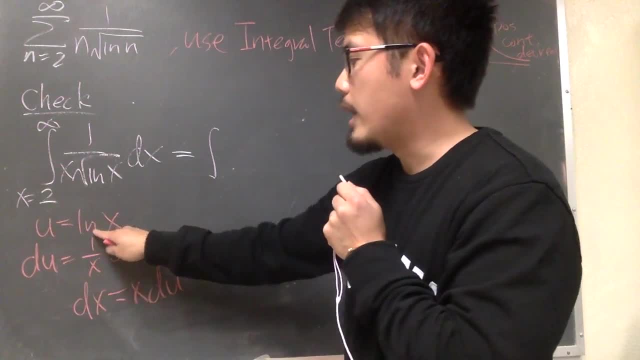 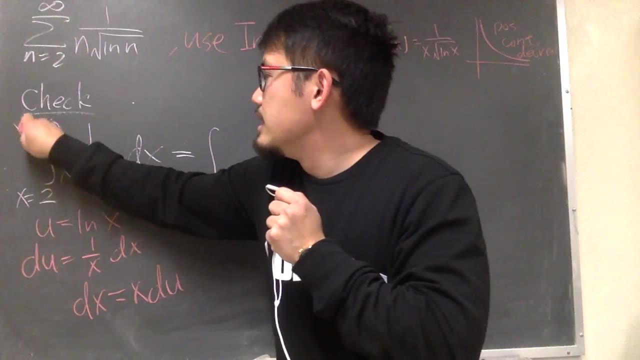 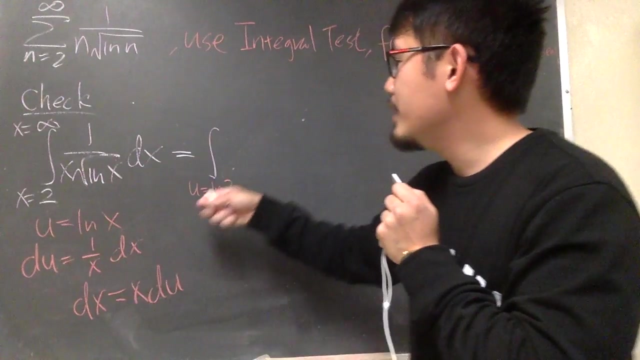 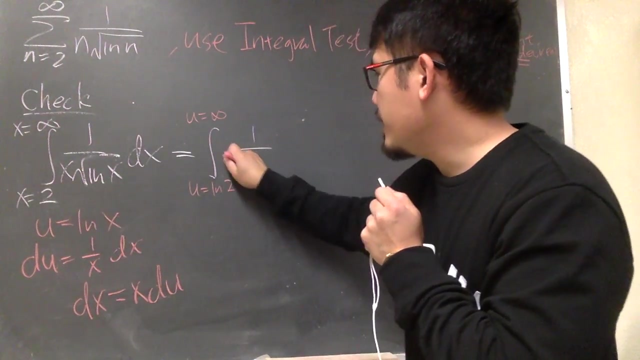 is equal to 2.. When x is equal to 2, that means u is equal to ln 2.. So in the u world, u is going from ln 2.. When x is infinity, we know ln of infinity, It's also infinity. u is also infinity. right here, Okay. And then inside we have 1 over. x is right. 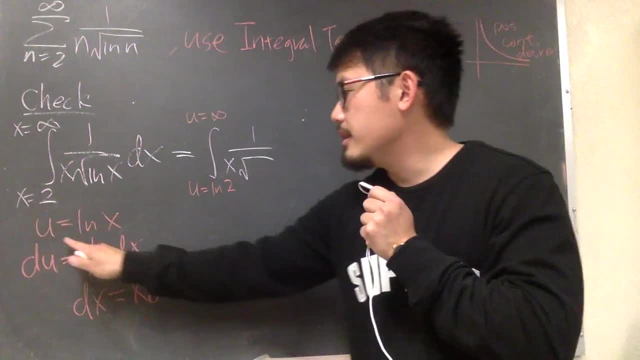 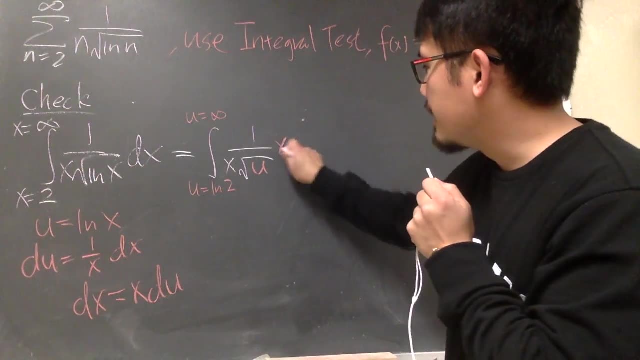 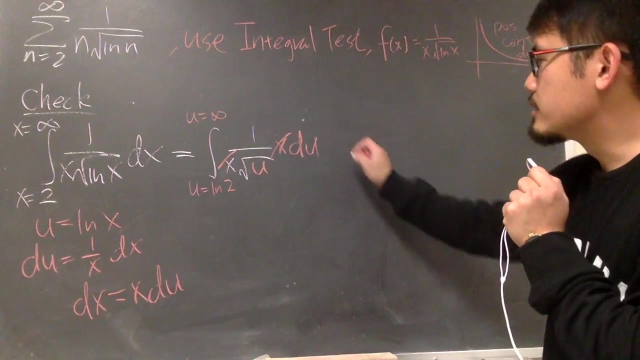 here Square root, the ln is the u, So I'll put down the u right here. dx is x times du, x times du, Like this, As we can see, this x and that x will cancel each other out. So now we can focus on. 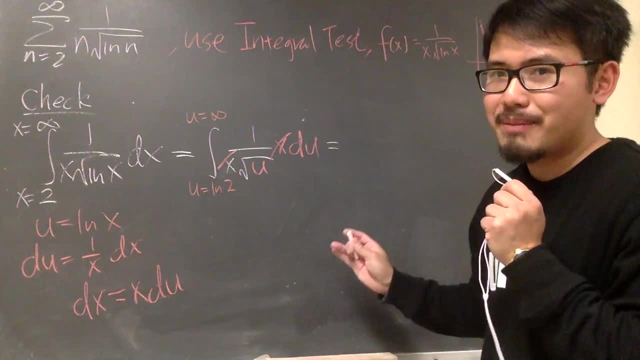 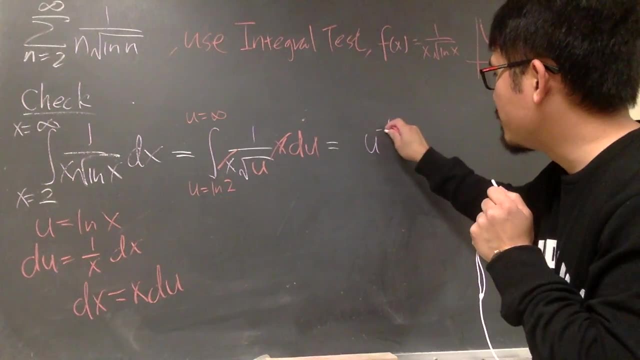 doing the integration, And to do so actually, you have to take one more step, 1 over square root of u. We are going to write it down as u to the negative 1 power first, Okay, And then we haven't done any integration yet. 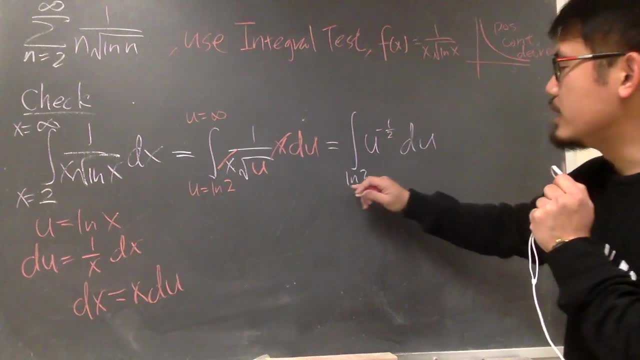 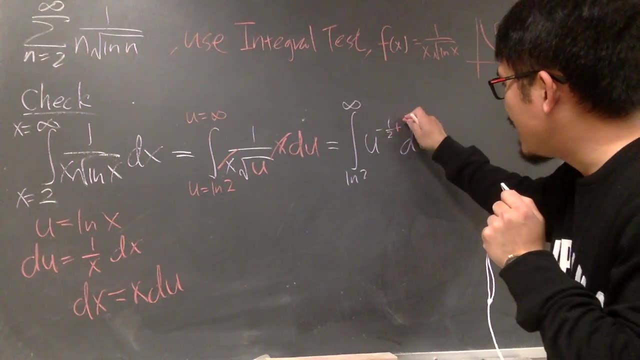 So we have to put this down. And then this is the u values: ln, 2 to infinity. How can we do this integral? Well, this is now power root backwards. We add 1 to it, Negative 1 plus 1. I mean negative. 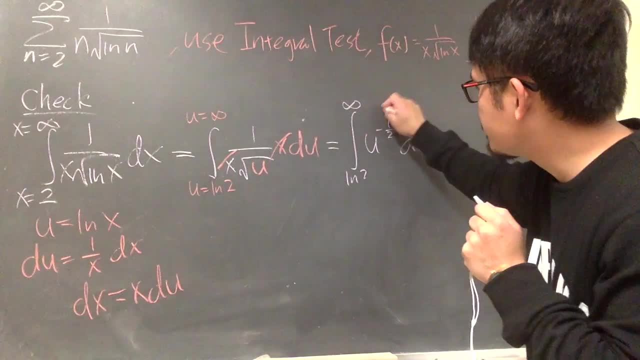 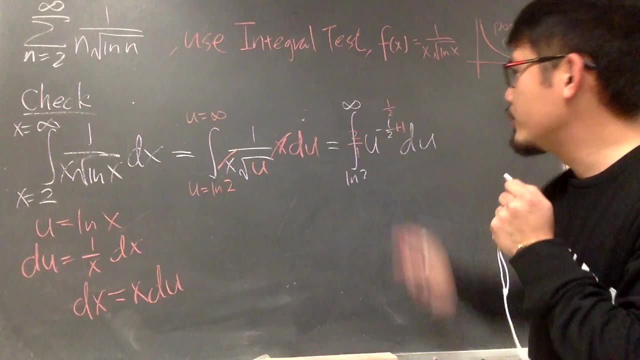 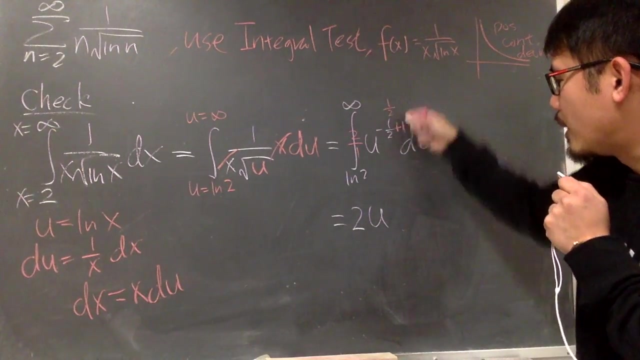 1 half plus 1.. It's positive 1 half, right. And then we have to divide it by this new power: Dividing by 1 half. it's the same as saying multiply by 2 over 1.. So now we have 2u, And this is the 1 half power.